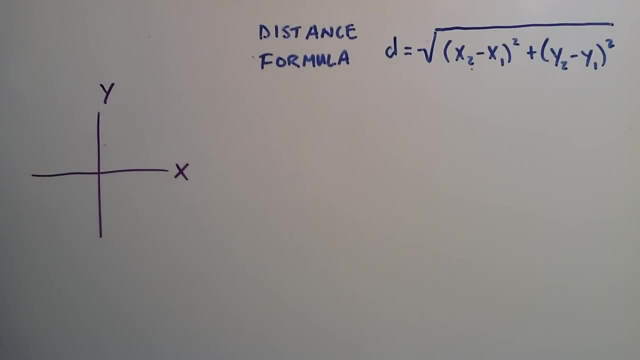 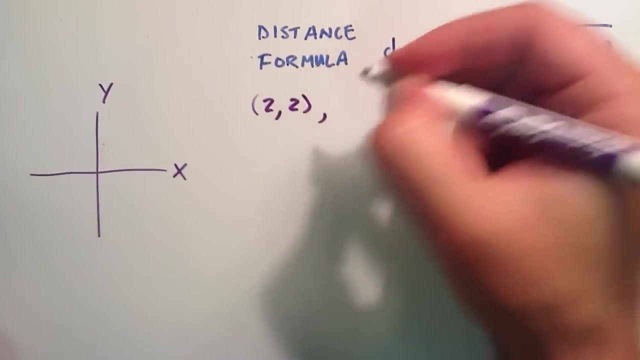 Hey everybody, this is Paul. Today I'm going to be showing you how to use the distance formula. So the distance formula tells us the distance between two points on an xy plane. So let's say that we have two points. Let's say the first point is 2, 2 and the second point is negative 2,. 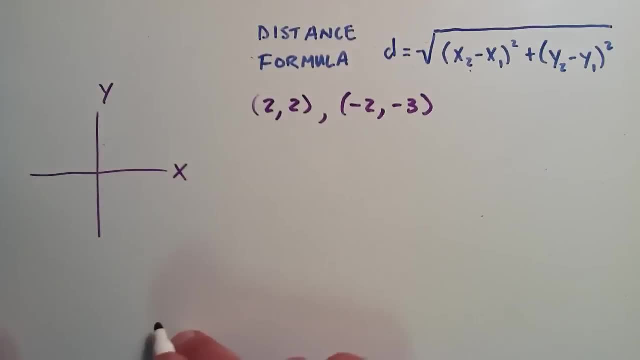 negative 3.. And we want to find the distance between these two points. So to get a visual understanding of this, let's go ahead and graph these. So the point 2, 2 is going to have an x component of 2 and a y component of 2.. So for the x component of 2, we start at the origin and move. 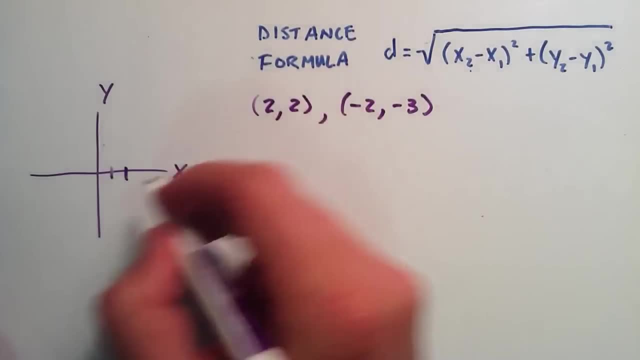 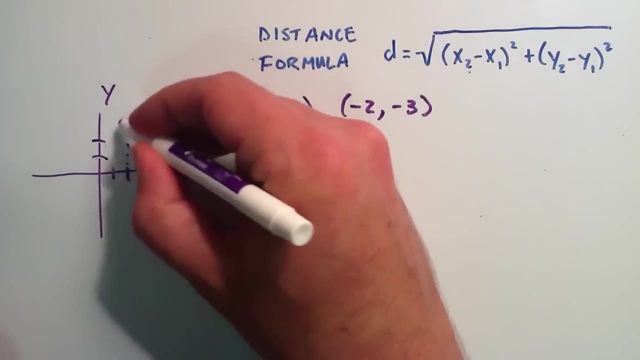 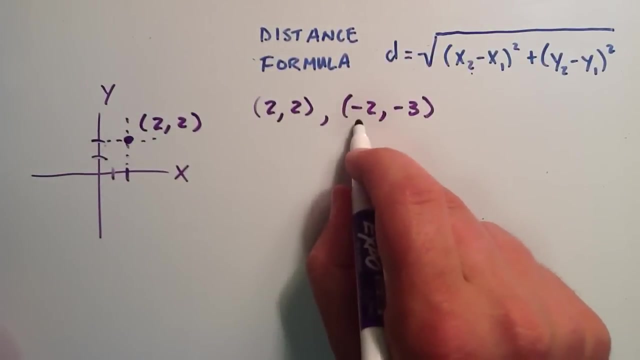 over 1, 2 units in the x direction. And for the y component of 2, we go up from the origin: 1, 2 units in the y direction, And then, where these little dotted lines cross right here, we have the point 2, 2.. And for our second point, 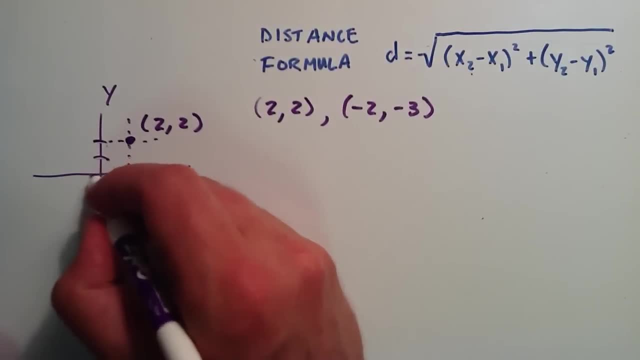 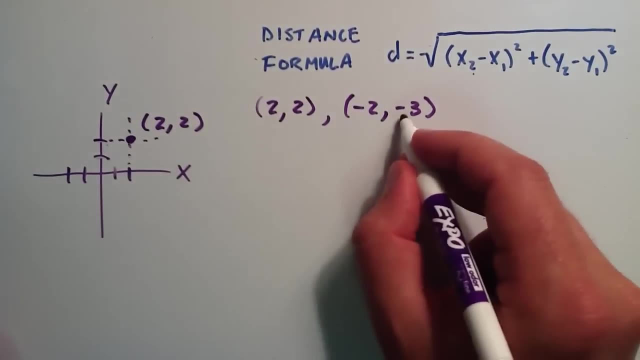 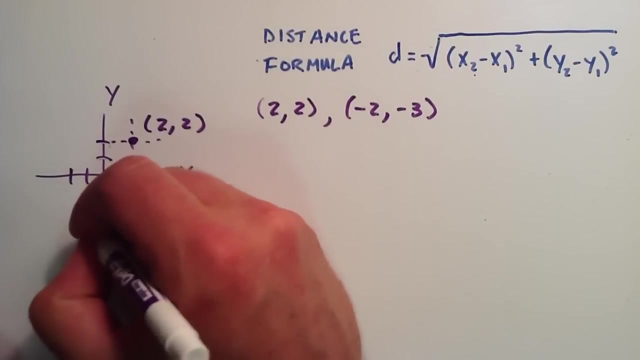 negative 2, negative 3.. Well, we just go: negative 1, negative 2 in the x direction, since negative 2 refers to the x component, And negative 3 in the y direction. Negative 1, negative 2, negative 3 for our y component of negative 3.. And where these two dotted lines cross, 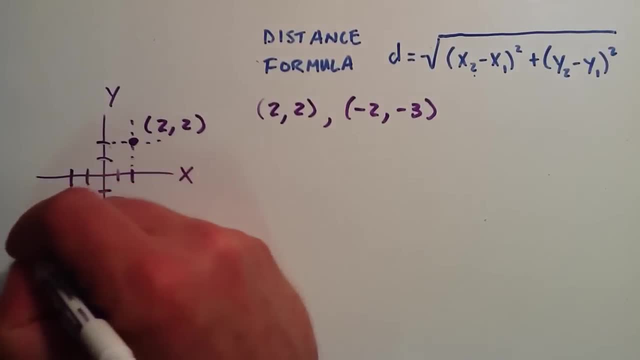 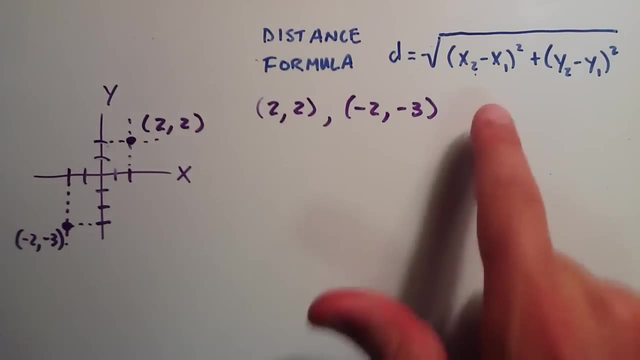 we have the point negative 2, negative 3.. So by plotting the distance between two points on an x plane we can get a visual understanding of the distance between two points on an x plane. So by plugging these two points into the distance, 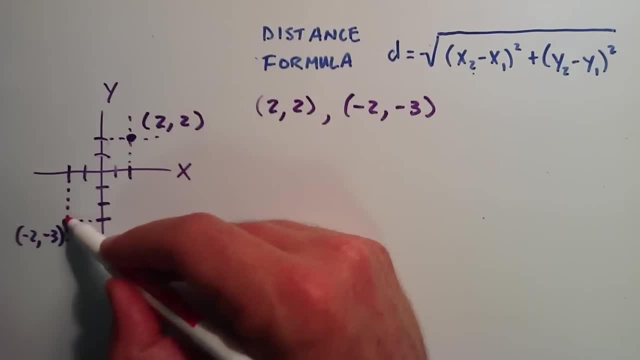 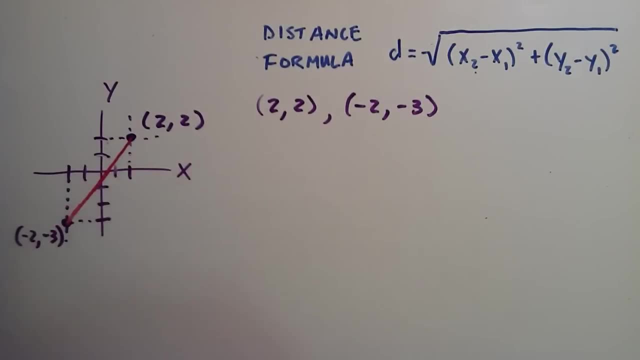 formula we're essentially going to find the length of the line that connects the two points or the line segment that connects the two points. So right now we just have some numbers in here. We don't have any x2,, x1s, y2s or y1s, So we're simply going to label one of these points: x1,, y1,. 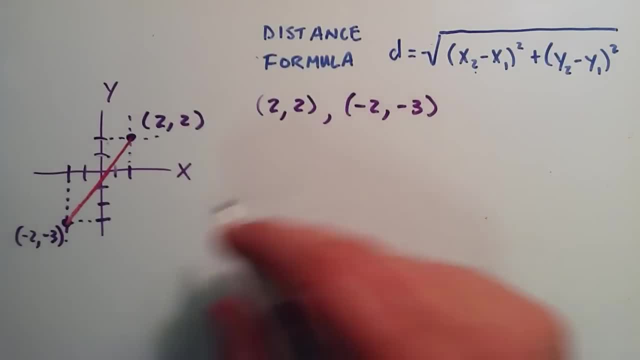 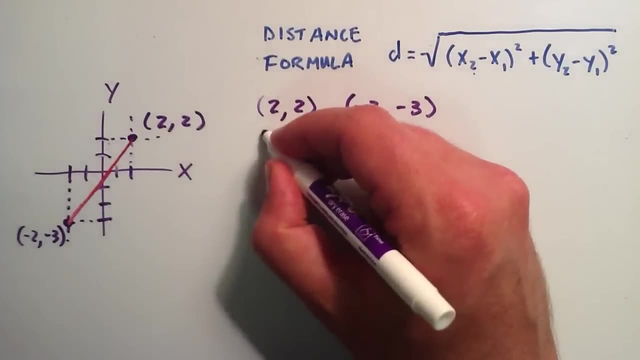 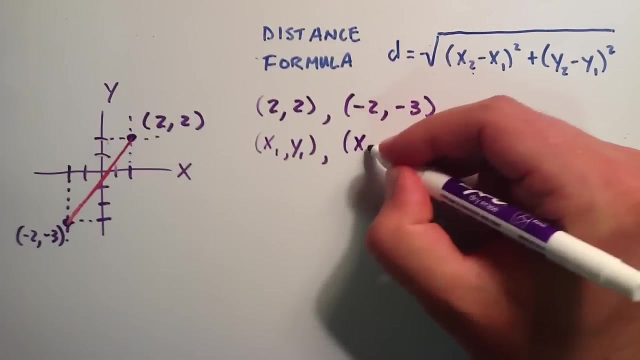 and the other one x2, y2.. And it doesn't matter which you choose to be which. if you plug them into the distance formula, you'll get the same answer. So we're just going to choose the first one to be x1, y1. And the second point we'll call x2, y2.. 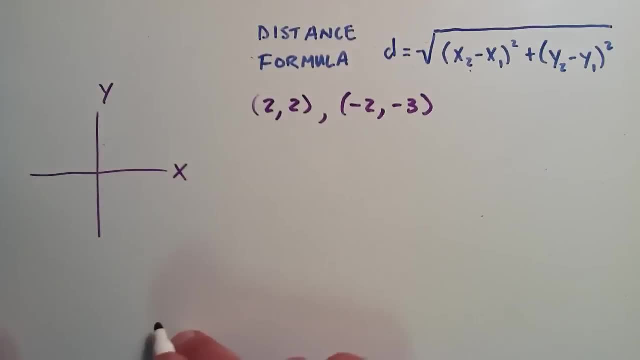 negative 3.. And we want to find the distance between these two points. So to get a visual understanding of this, let's go ahead and graph these. So the point 2, 2 is going to have an x component of 2 and a y component of 2.. So for the x component of 2, we start at the origin and move. 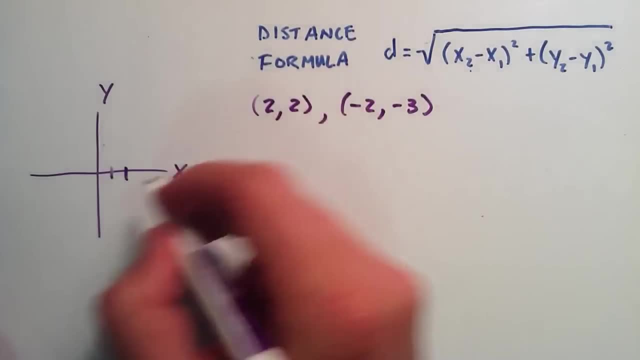 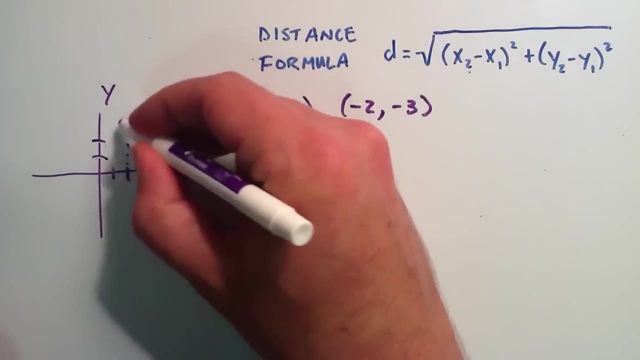 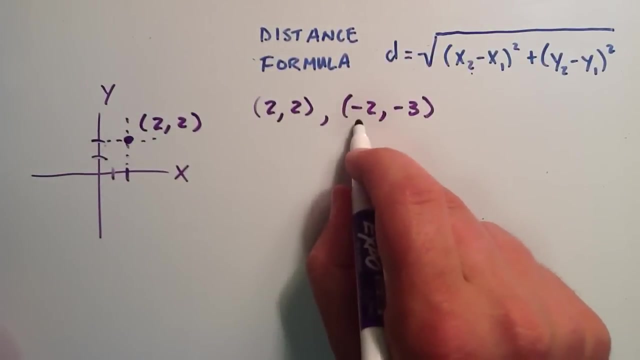 over 1, 2 units in the x direction. And for the y component of 2, we go up from the origin: 1, 2 units in the y direction, And then, where these little dotted lines cross right here, we have the point 2, 2.. And for our second point, 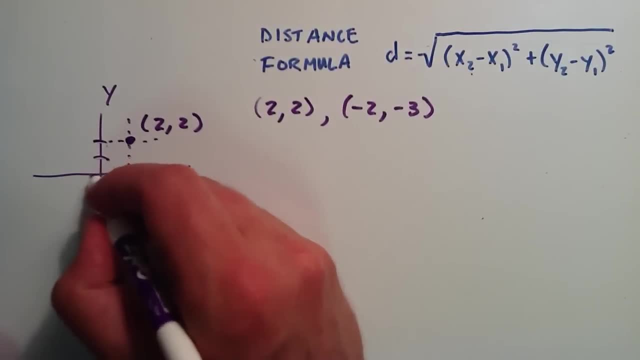 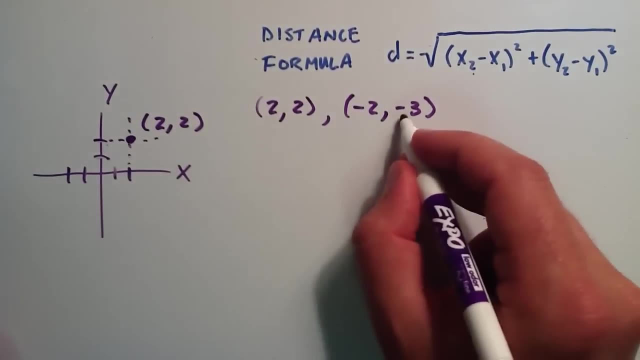 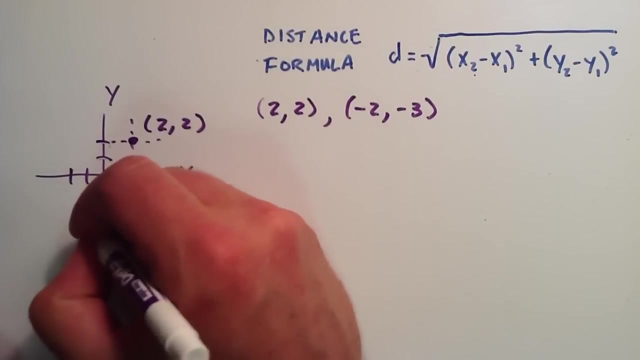 negative 2, negative 3.. Well, we just go: negative 1, negative 2 in the x direction, since negative 2 refers to the x component, And negative 3 in the y direction. Negative 1, negative 2, negative 3 for our y component of negative 3.. And where these two dotted lines cross, 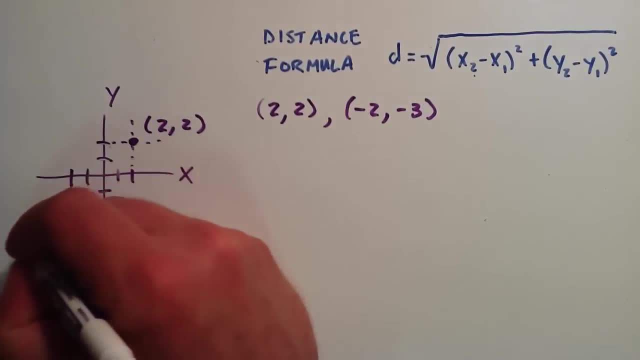 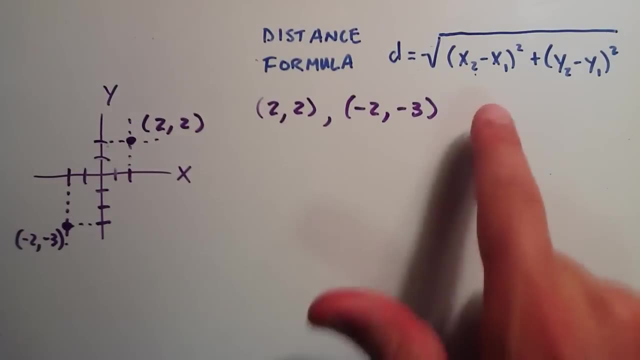 we have the point negative 2, negative 3.. So by plotting the distance between two points on an x plane we can get a visual understanding of the distance between two points on an x plane. So by plugging these two points into the distance, 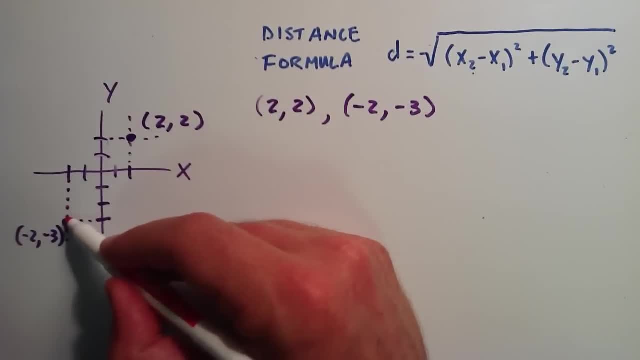 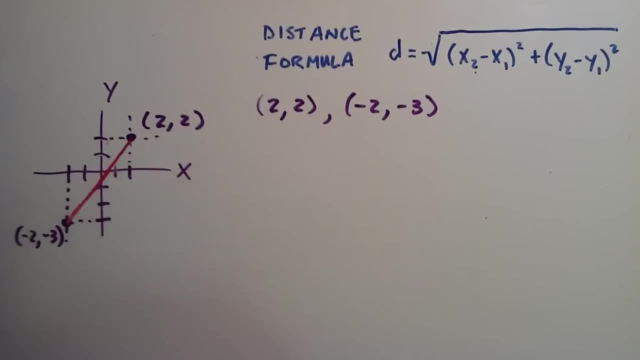 formula we're essentially going to find the length of the line that connects the two points or the line segment that connects the two points. So right now we just have some numbers in here. We don't have any x2,, x1s, y2s or y1s, So we're simply going to label one of these points: x1,, y1,. 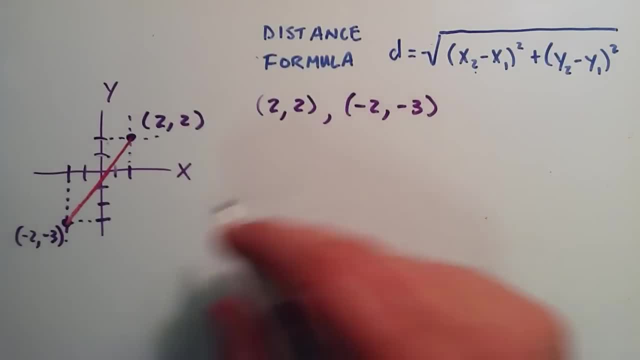 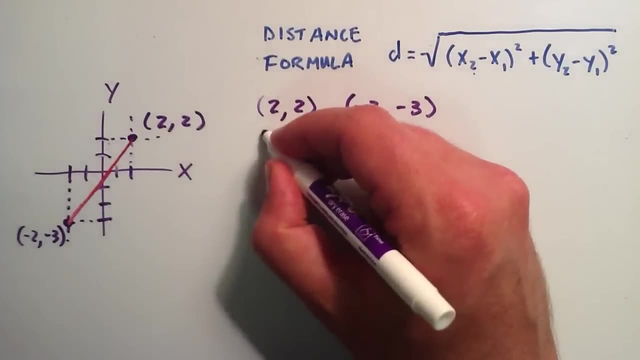 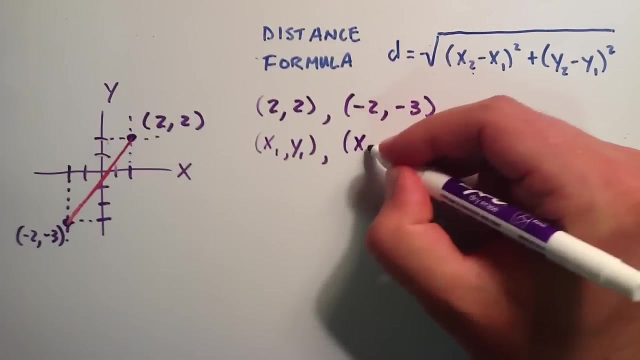 and the other one x2, y2.. And it doesn't matter which you choose to be which. if you plug them into the distance formula, you'll get the same answer. So we're just going to choose the first one to be x1, y1. And the second point we'll call x2, y2.. 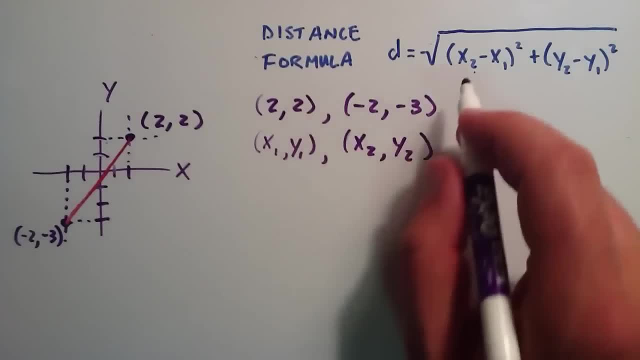 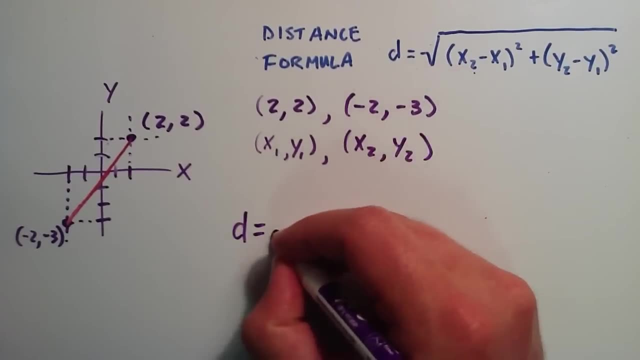 And we simply plug in these numbers where they correspond in the distance formula. So the distance of this red line that I just drew is simply equal to the square root, And then we just plug in the distance formula And we simply plug in the distance formula. 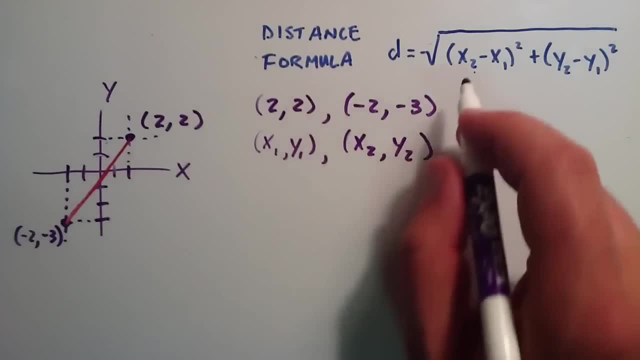 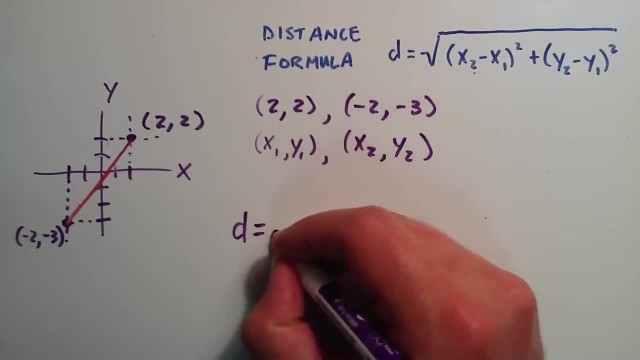 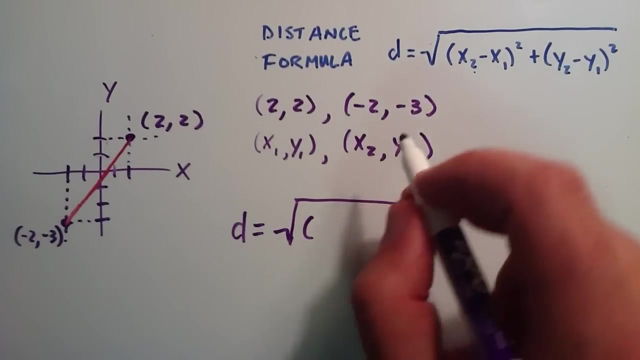 And we simply plug in these numbers where they correspond in the distance formula. So the distance of this red line that I just drew is simply equal to the square root. So we need x2 minus x1.. So x2 is equal to negative 2. It corresponds to the left-hand side of this. 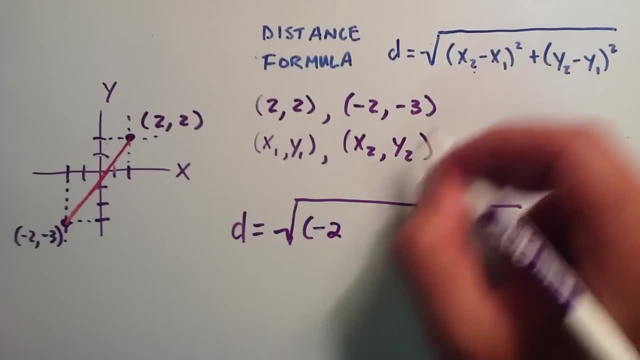 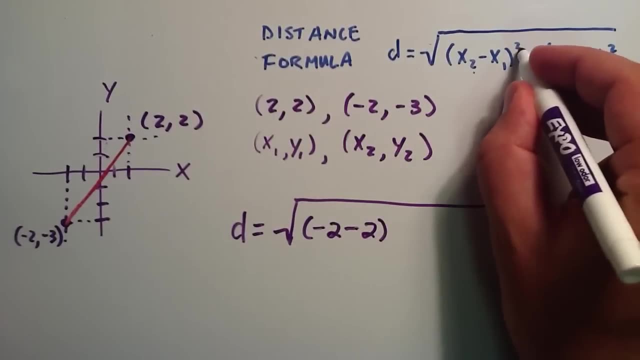 point, So negative 2.. And then we're subtracting x1.. So we subtract, x1 corresponds to the left-hand side of this point, which is a 2. And then that's squared, And then we add that to y2,. 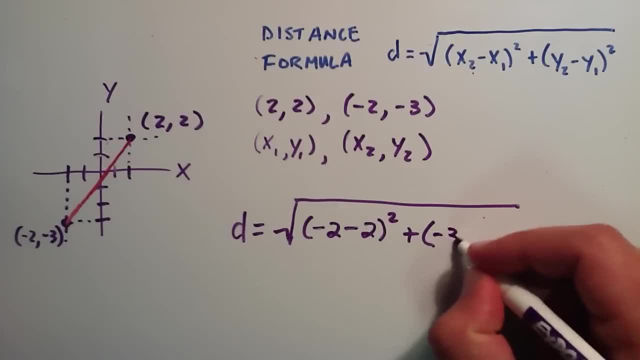 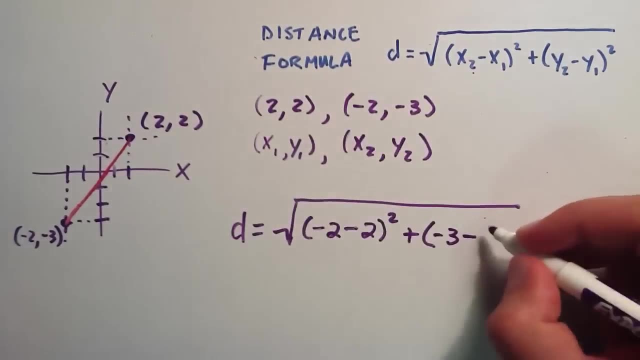 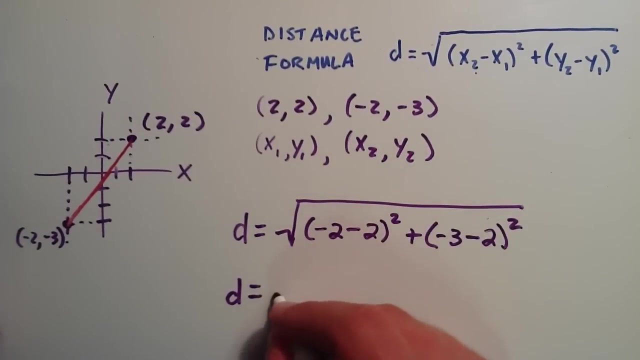 which is the right-hand side of this point. So that's a negative 3.. And we subtract y1.. And y1 corresponds to the right-hand side of this point, which is a 2.. So the distance between those two points is simply the square root of negative 2 minus. 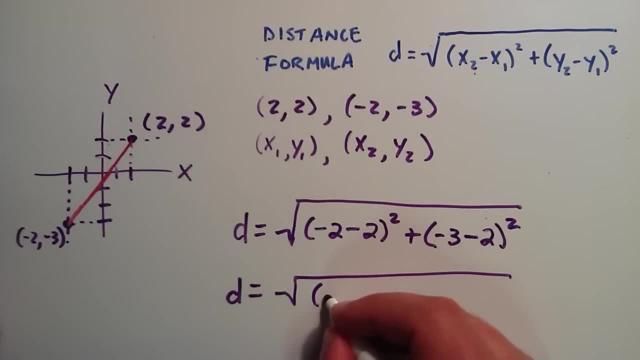 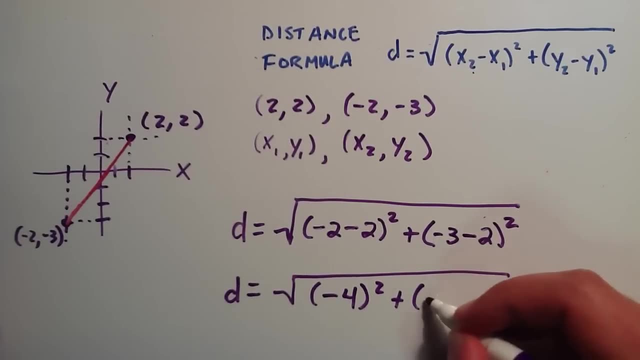 2 squared And negative 2. take away another 2 squared is negative 4 squared plus negative 3 minus 2, which is a negative 5 squared. And so now negative 4 squared is the same thing as negative 4 times negative 4, which 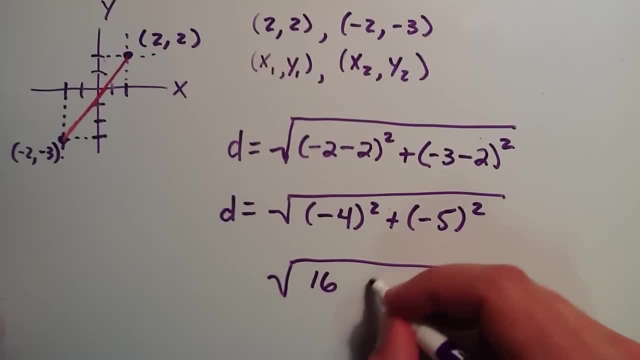 is 16.. And negative 5 squared is the same thing as negative 5 times negative 5, or 25.. And 16 plus 25 is 41. So the distance between the point 2, 2 and negative 2, negative 3 is: 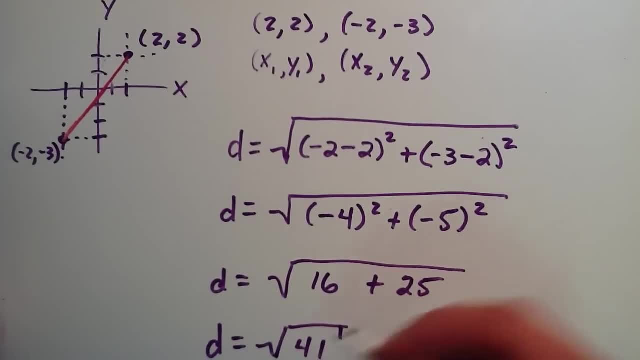 simply 4 squared, And so now negative 4 squared is the same thing as negative 4 times negative 4, which is a negative 6 squared, And thisιm a square root of 41. So square root 41 is the length of this line and that 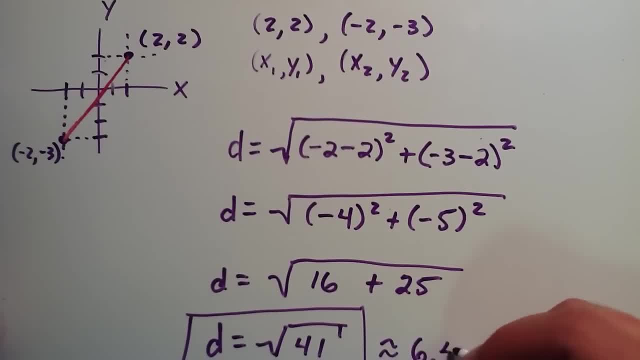 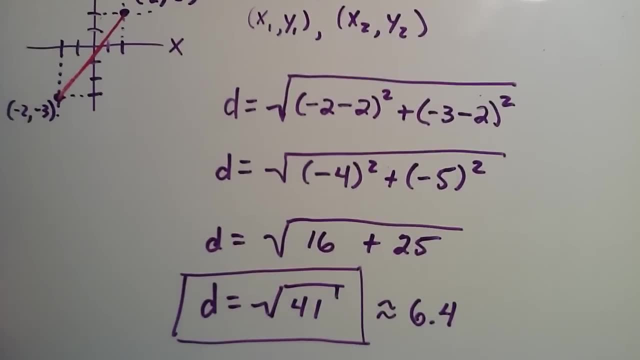 is approximately equal to 6.4.. So the distance between these two points is about 6.4.. If you want an exact answer, then write it in this form: square root 41.. This is the exact distance. This is an approximate. 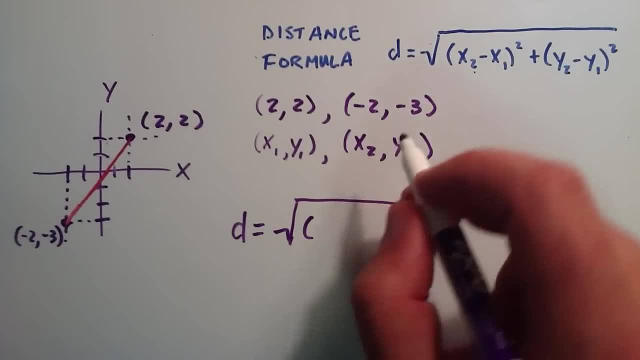 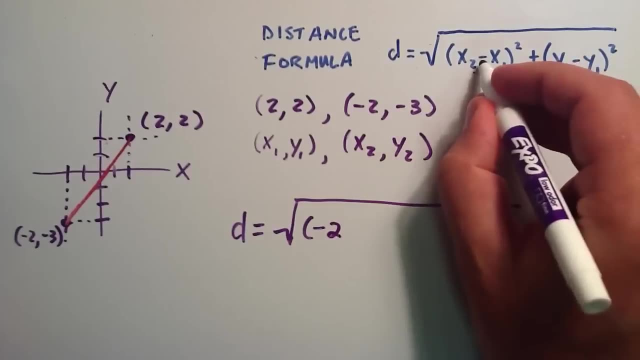 So we need x2 minus x1.. So x2 is equal to negative 2. It corresponds to the left-hand side of this point. So negative 2.. And then we're subtracting x1.. So we subtract, x1 corresponds to the left-hand. 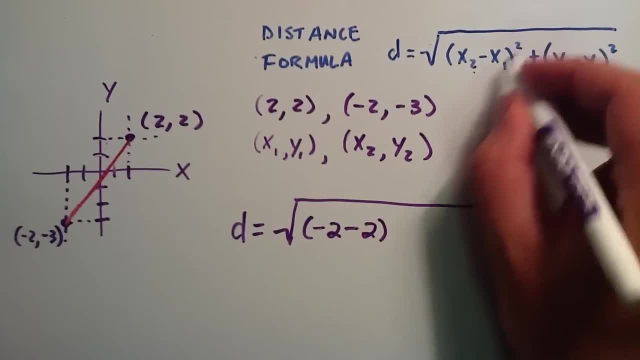 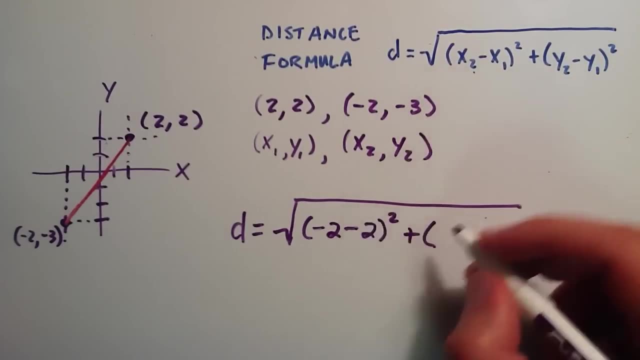 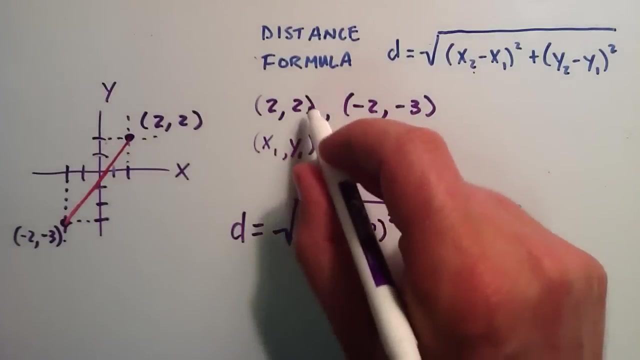 side of this point, which is a 2.. And then that's squared, And then we add that to y2, which is the right-hand side of this point, So that's a negative 3. And we subtract y1. And y1 corresponds to the right-hand side of this point, which is a 2.. 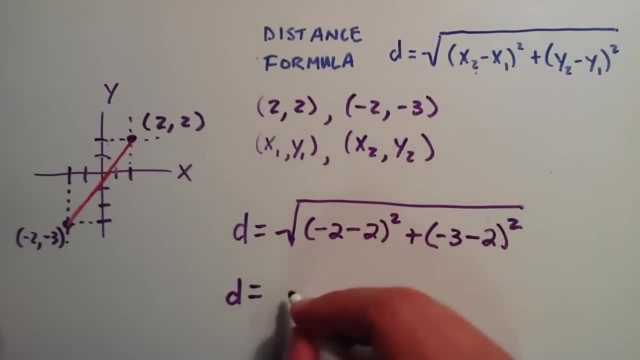 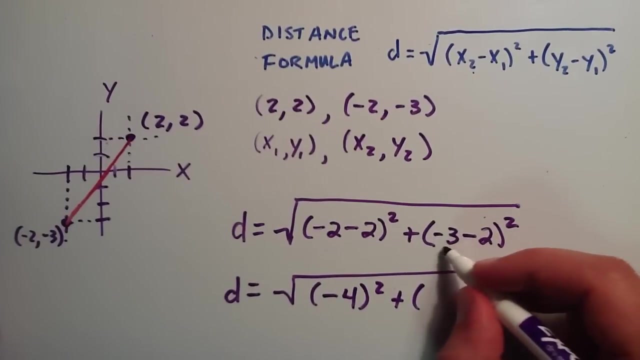 So the distance between those two points is simply the square root of negative 2 minus 2 squared And negative 2, take away another 2 squared is negative 4 squared, plus negative 3 minus 2, which is a negative 5 squared. 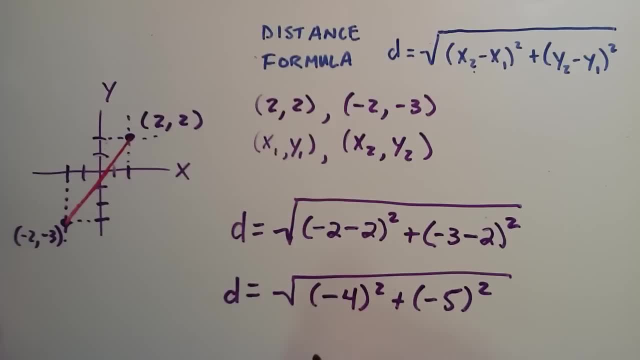 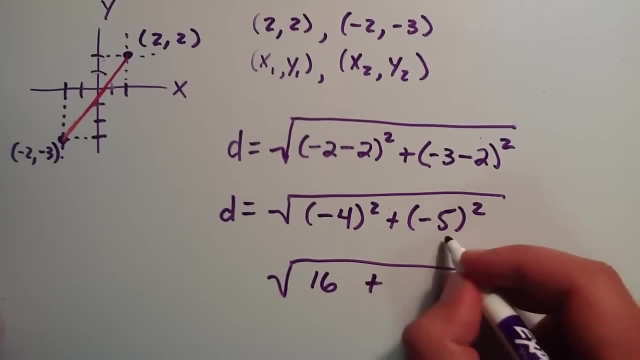 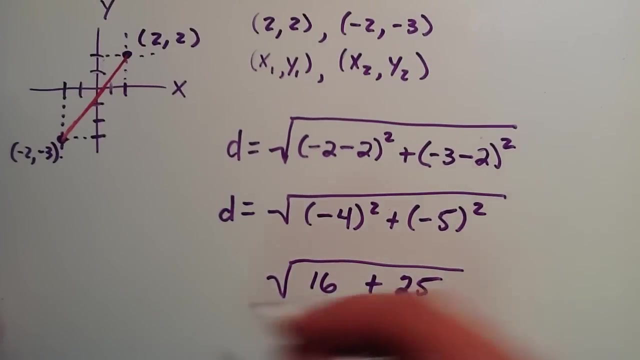 And so now negative 4 squared is the same thing as negative 4 times negative 4, which is 16.. And negative 5 squared is the same thing as negative 5 times negative 5, or 25.. And 16 plus 25 is 41. So the distance between the point 2, 2 and negative 2, negative. 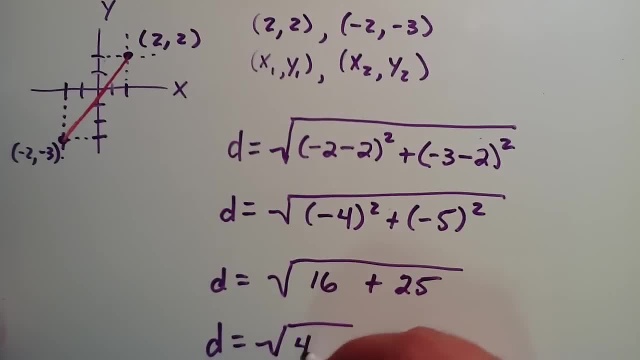 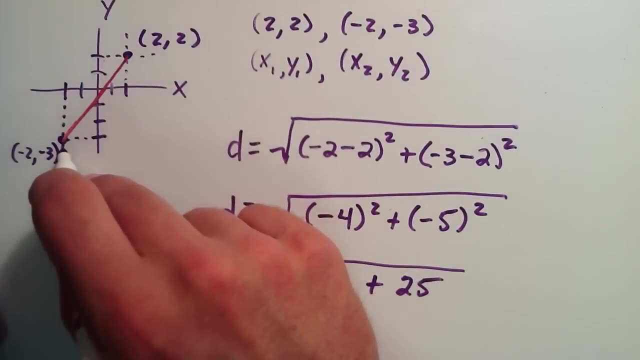 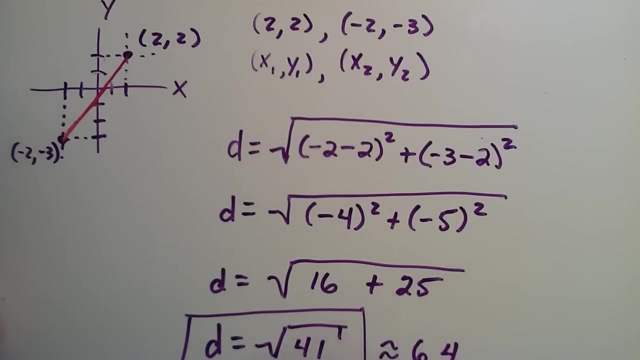 3 is simply the square root of negative 3.. And so now negative 4 squared is the same square root of 41.. So square root of 41 is the length of this line, And that is approximately equal to 6.4.. So the distance between these two points is about 6.4.. If you want an exact 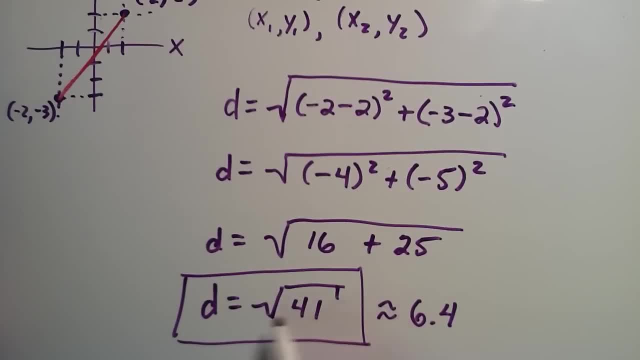 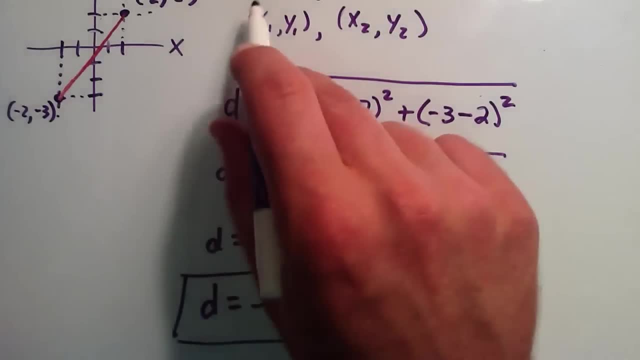 answer, then write it in this form: Square root of 41,. this is the exact distance, This is an approximate distance, And so we right-wing this equation And we can also write: 지금, between the points 2, 2 and negative, 2, negative 3.. 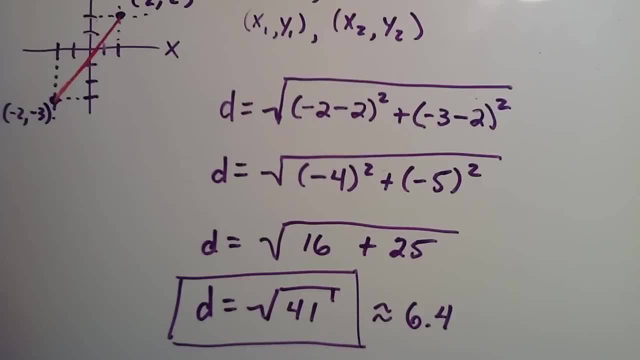 Hopefully you've enjoyed this tutorial and don't forget to subscribe. 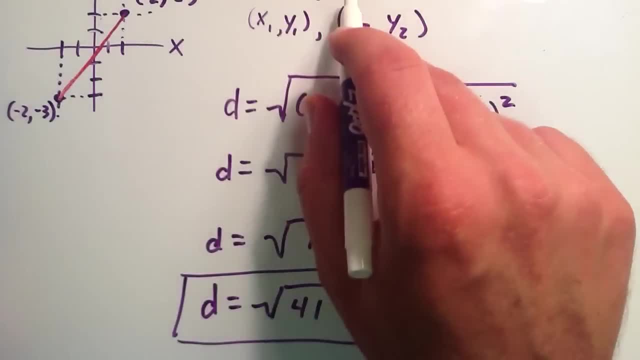 distance between the points and Hopefully you've enjoyed this tutorial and don't forget to subscribe.